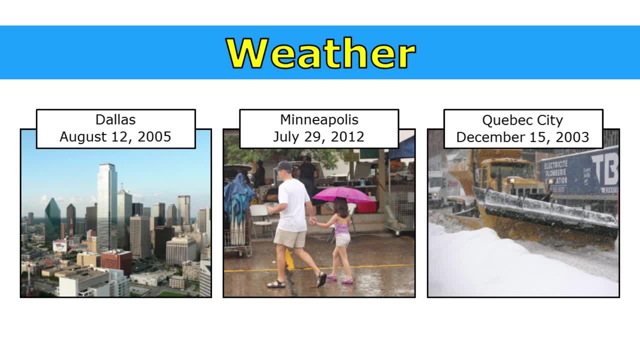 In Minneapolis on July 29, 2012,. it was warm and raining, And in Quebec City on December 15, 2003,. it was cold and snowing. These are all descriptions of the weather In these locations on these specific days. 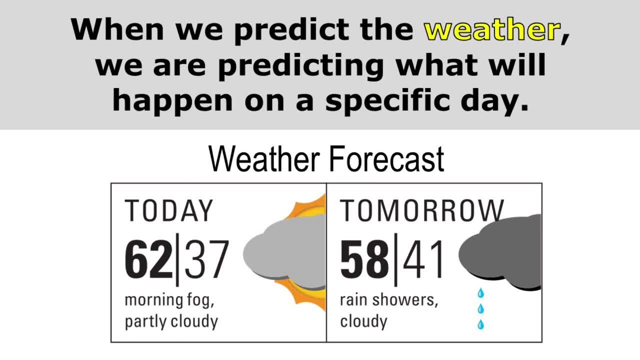 When we predict the weather, we are predicting what will happen on a specific day, And another word for prediction is forecast, And so our weather forecast is our prediction of what will happen in the weather on a specific day. So sometimes we even talk about what might happen not just on the day as a whole, but 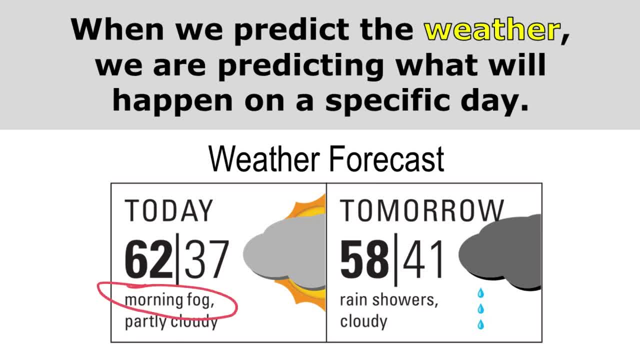 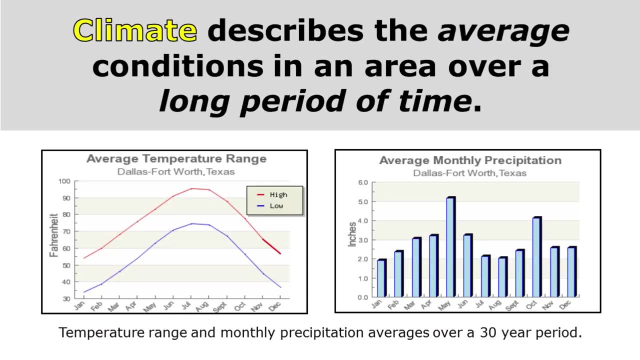 what might happen in the morning, like here Predicting morning fog- or in the evening, Maybe there will be evening showers. And so, as we predict what will happen at specific times on specific days, we're predicting the weather. Climate is different than weather. 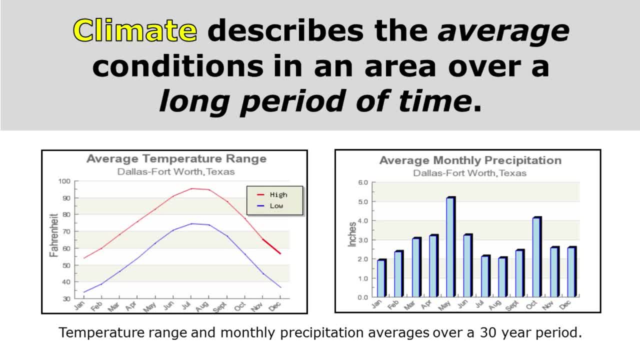 Climate describes the average conditions in an area over a long period of time, And you see these two graphs here. They're about the average temperature and the average monthly precipitation over a 30-year period. It's the average temperature in the Dallas-Fort Worth area. 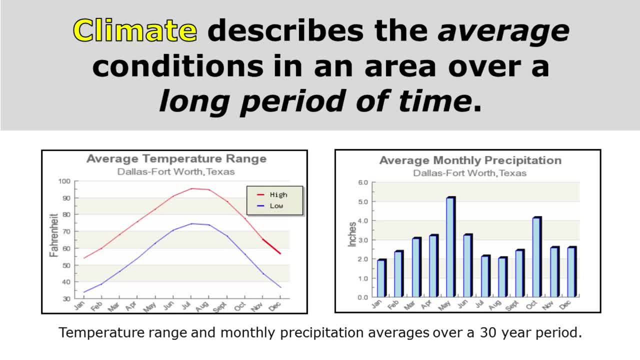 And so these aren't what happened on a specific day. This is an average of what happened over a very long period of time. So when I look at this data, I can see that the highest average temperatures happen in the month of July. That doesn't tell me exactly what the temperatures will be on any specific days in July, but 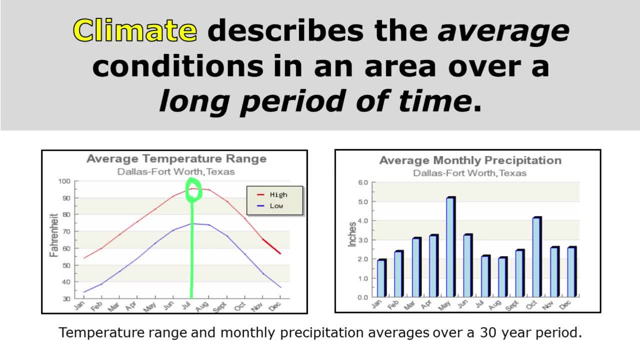 it does tell me that I can expect July to be a very warm month. look at the other bar graph about precipitation. I can see that May and October have experienced the most rain over the last 30 years. Once again, that doesn't tell me what days it's going to rain next May or next October, but it 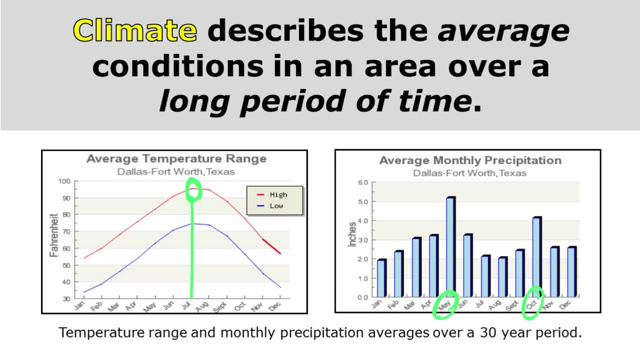 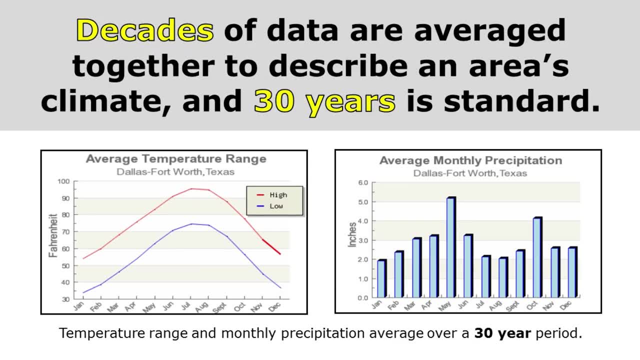 does tell me that I should expect more rain in those months next year than I'll probably get in August or December. Decades of data are averaged together to describe an area's climate, and 30 years is standard, And these two graphs are actually the temperature range and monthly precipitation averages over a